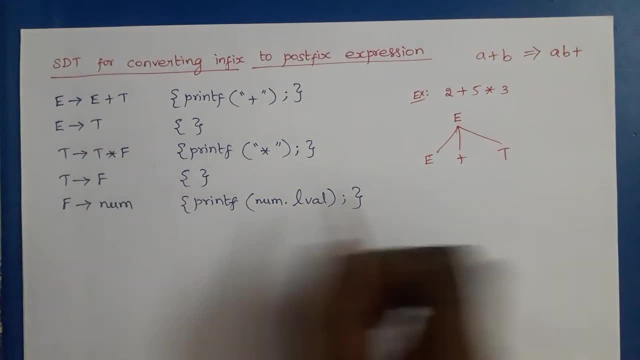 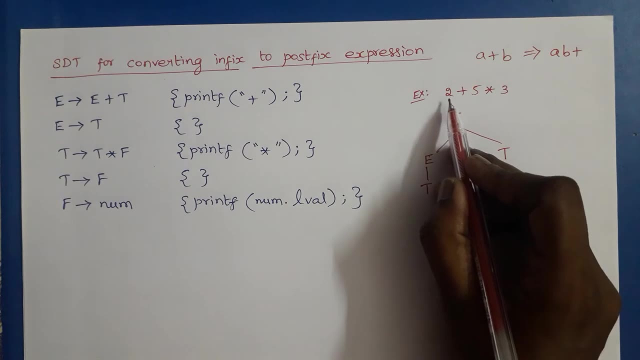 E is a start symbol of the grammar. E can be expanded by using any one of these two predictions. so we need addition expression. So E can be expanded by using e plus t. then this E can be expanded by using t. Since we need 2 before plus, we need single number. so e can be expanded by using t. t tends to f, f tends to number. 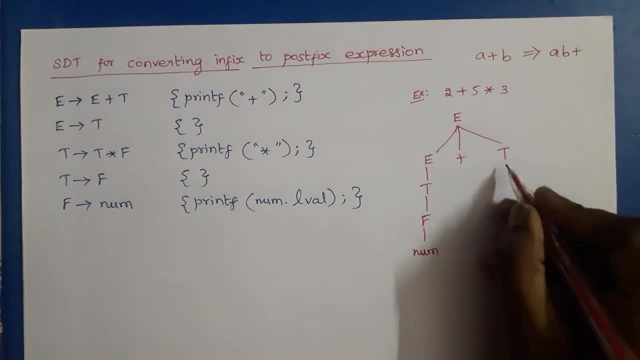 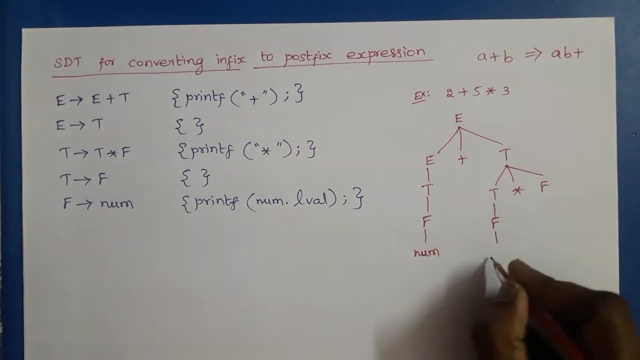 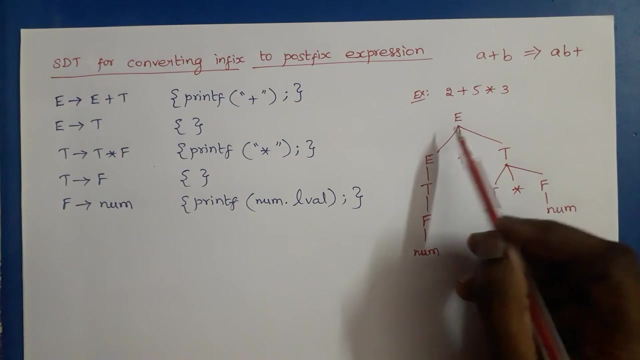 number. then this t can be expanded by using t star f, because after the plus we need multiplication expression. so t star f. then this t can be expanded by using f. then f tends to number, then this f tends to number. so now we have to find the semantic actions for converting. 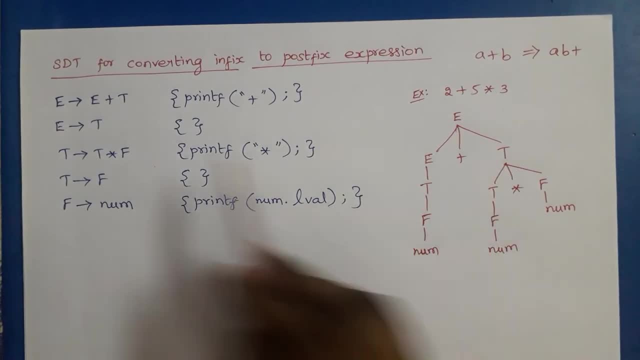 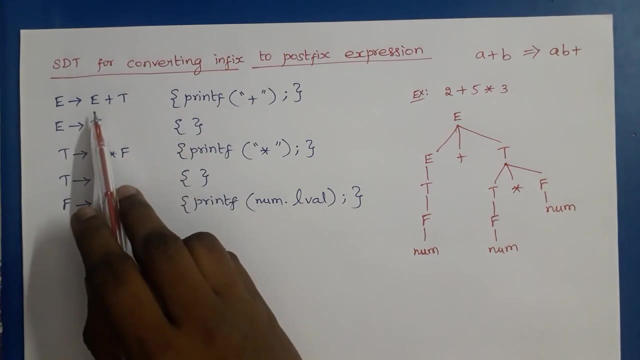 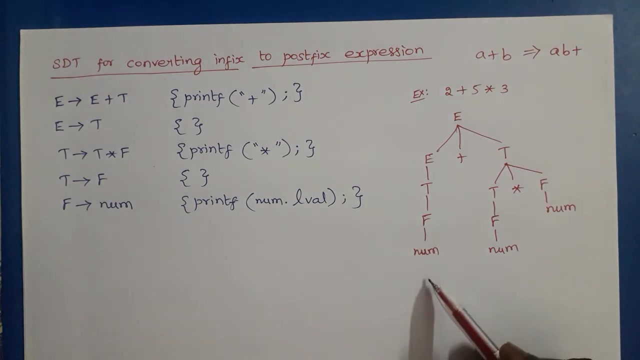 this infix into postfix, so e tends to e plus t. so after reducing e and t only we can execute the semantic action. so now this e is expanded by using t, so e tends to t, then t tends to f and f tends to number. that is in bottom up fashion. we are going to assign the, we are 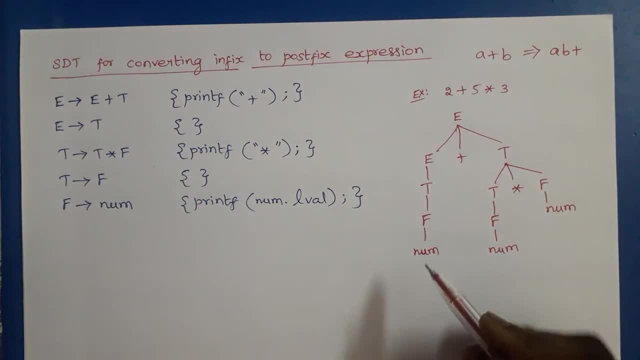 going to execute the semantic action. so we will reach the number here. f tends to number. so what is the semantic action associated with the f tends to number printf numlval. so what is the lexical value for this number? actually, this number is 2, this one is 5 and this is 3, so the postfix notation is first: f tends to number will be: 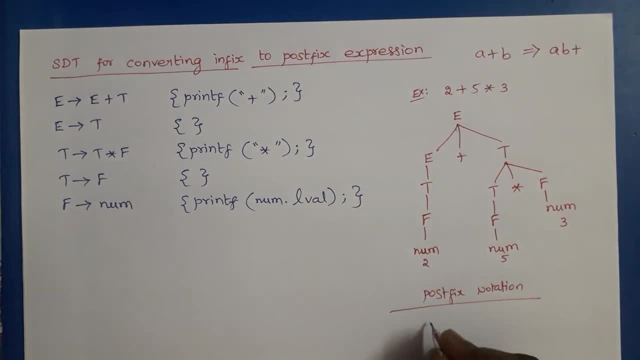 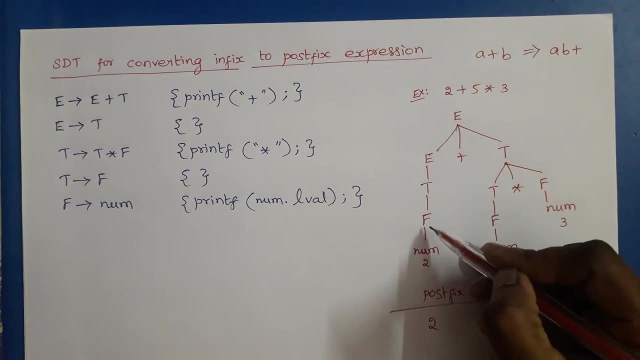 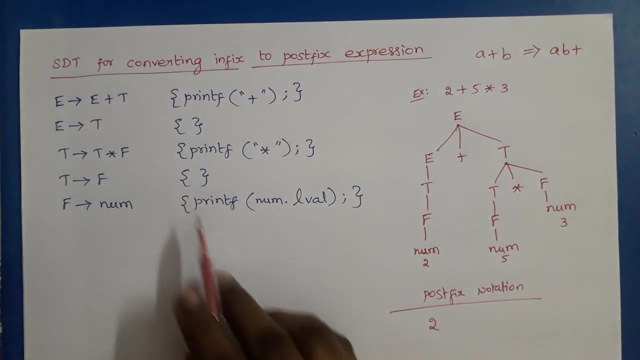 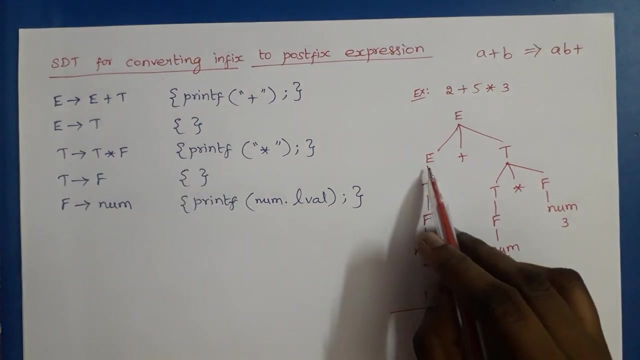 executed. so printf numlval. so this 2 will be printed. then t tends to f, t tends to f. so what is the semantic action for t tends to f? no action, so nothing will be performed here. then e tends to t. here also there is no semantic action. 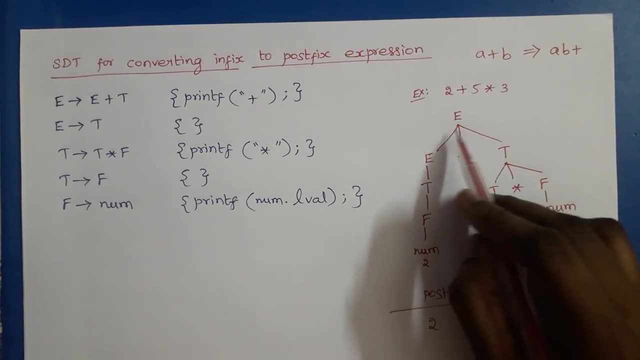 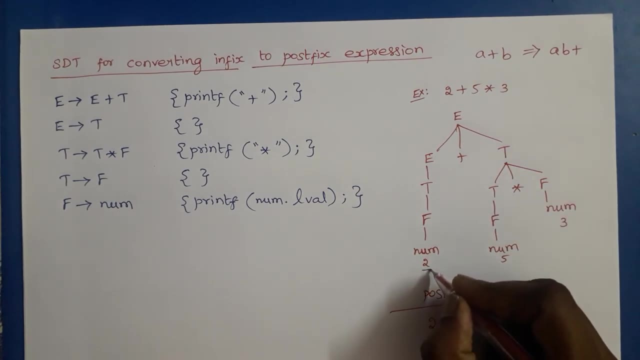 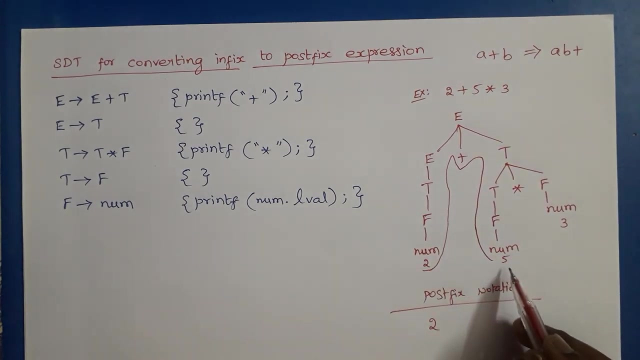 then before executing semantic action for e tends to e plus t, we need to go here because in bottom up fashion, after the e tends to t, we are going to execute the semantic action for e tends to e plus t. so after this we should come over here. so 5 in 5 is a num value, so f tends to num printf.